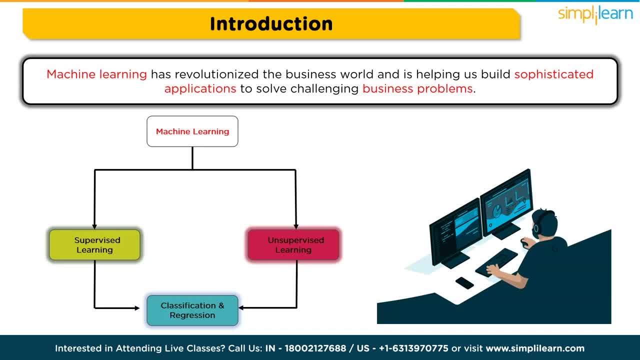 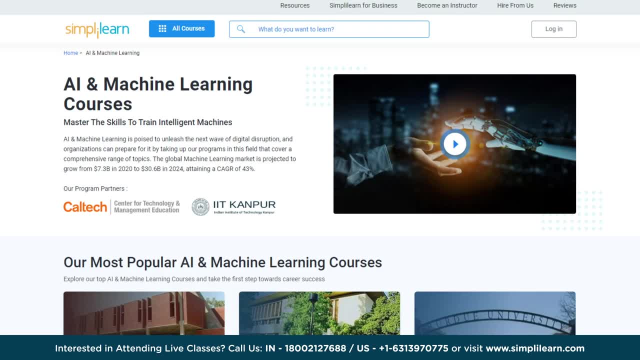 machine learning algorithm in Python called logistic regression. Logistic regression can be used to solve both classification and regression problems. Just a quick info for you. if you want to upskill yourself, master AI and machine learning skills and land your dream job or grow in your career, then you must explore Simply. 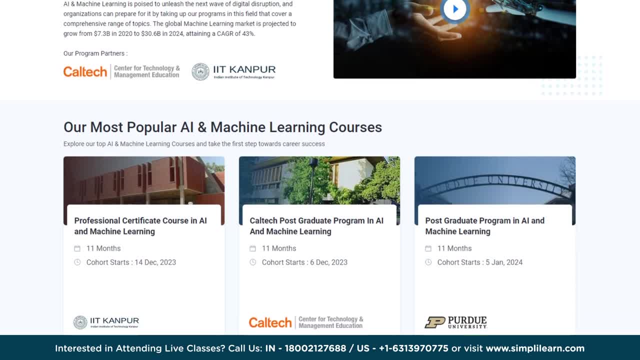 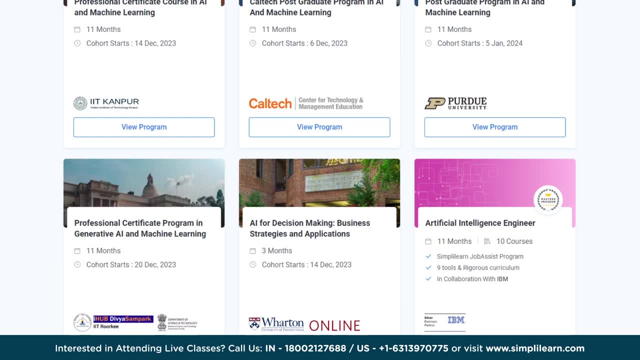 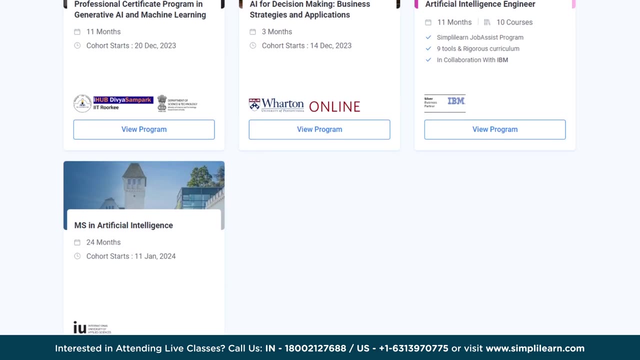 Learn's cohort of various AI and ML programs. Simply Learn offers various certification and postgraduate programs in collaboration with some of the world-leading universities like Wharton, Purdue, Caltech and Stanford. Through our courses, you will gain knowledge and work-ready expertise in skills like generative 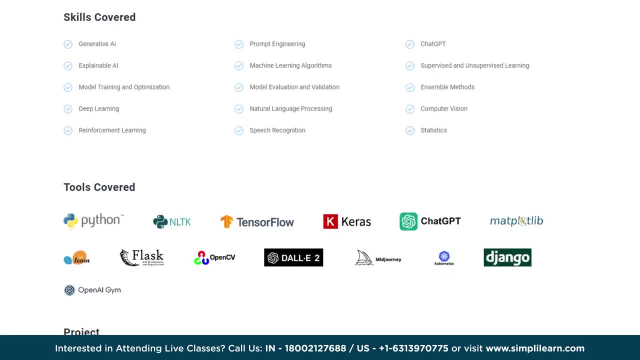 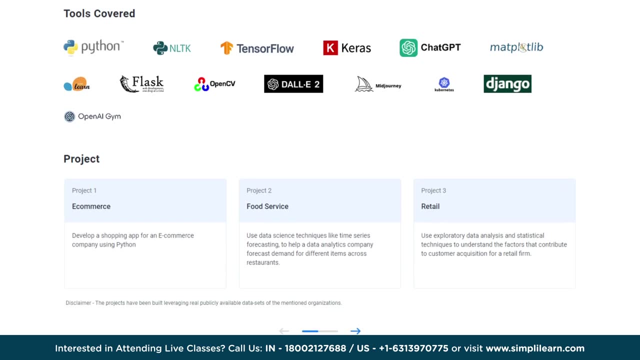 AI, prompt engineering, explainable AI, machine learning algorithms and over a dozen others. That's not all. You also get the opportunity to work on multiple projects and learn from industry experts working in top tier product companies and academicians from top universities. 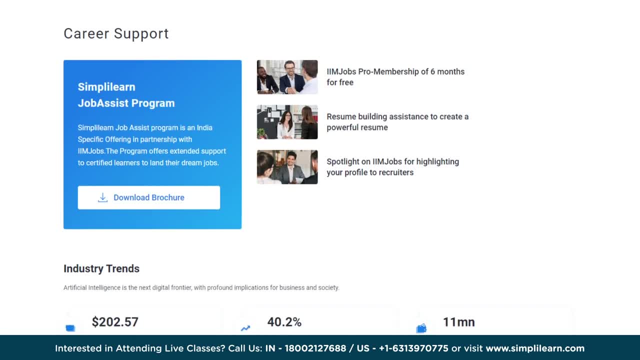 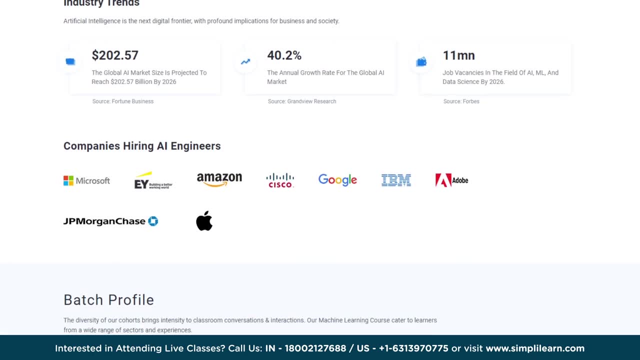 After completing these courses, thousands of learners have transitioned into an AI or ML role. If you are a passionate about making your career in this field, then make sure to check out the link in the pinned comment and the description box to find an AI or ML program. 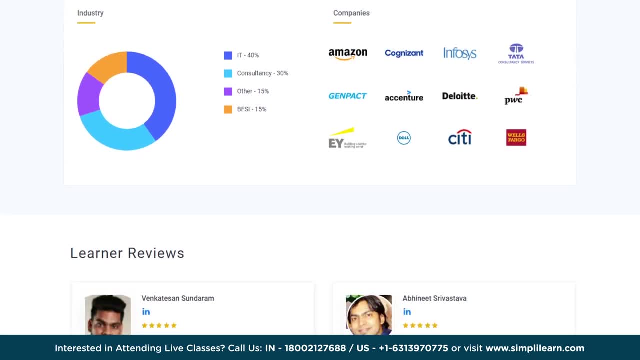 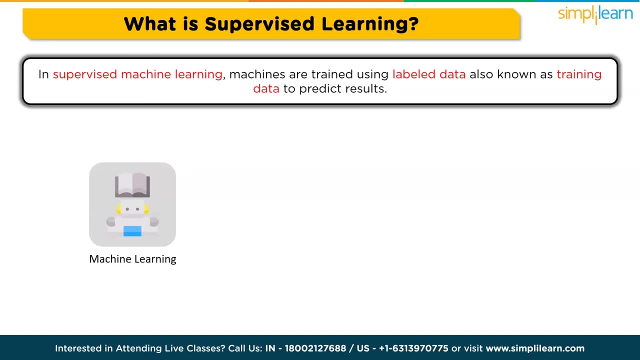 that fits your experience and areas of interest. So, moving forward, let's take a quick look at supervised learning. What is supervised learning? In supervised machine learning, machines are trained using labeled data, also known as training data, to predict results. Here, labeled data refers to a group of data have been tagged. 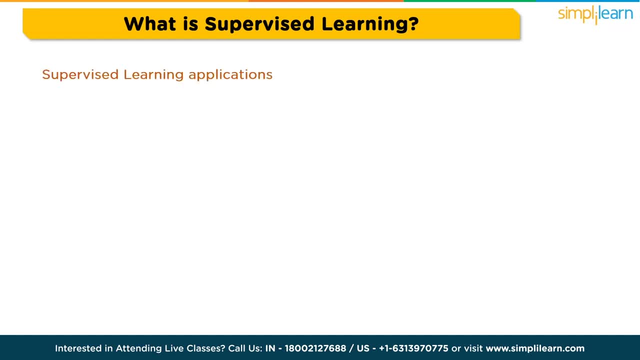 into one or more names and the data is already known to the machine. In the real world. supervised machine learning can be used for image object detection, predictive analytics, spam detection and customer sentiment analysis and many more. Supervised learning problems can further be classified into regression and classification. 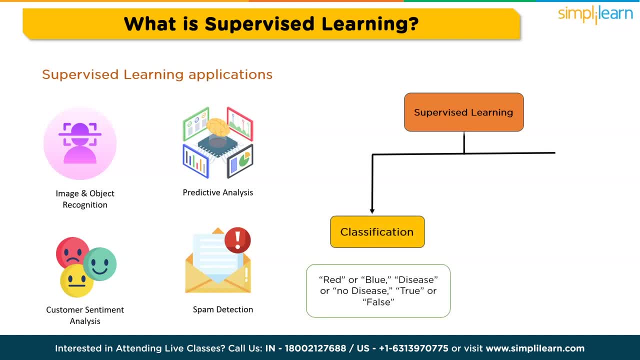 problems. In classification problems, the output variable is a category, such as red or blue disease or no disease, true or false and many others. In regression problems, the output variable is the real name. The problem is classified into a row. 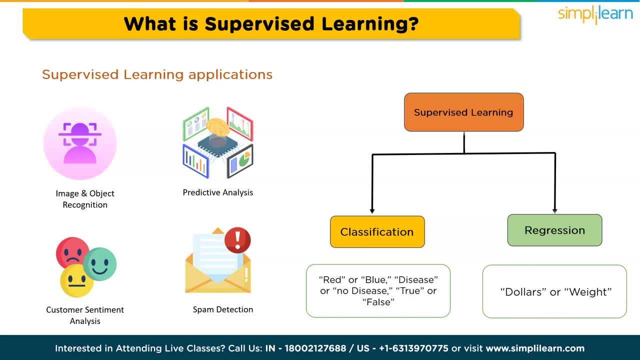 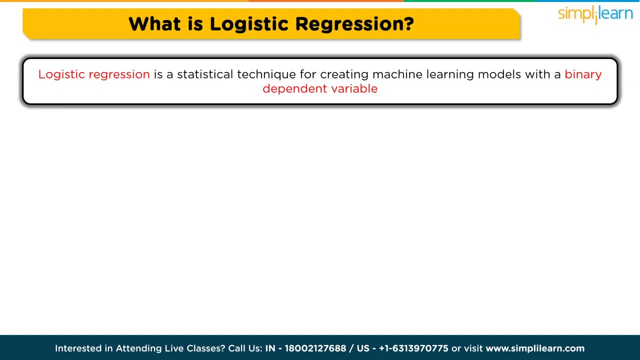 In regression problems, the output variable is the real name, The problem is classified real continuous value, such as dollars or weight. So now let's move forward and have a look on what is logistic regression. Logistic regression is a statistical technique for creating machine learning. 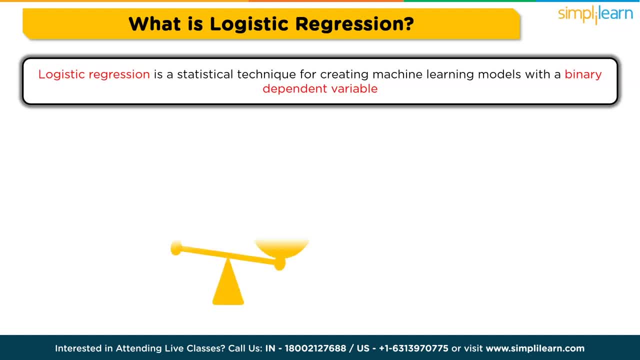 models with a binary of dependent variable. It describes the relationship between two variable, dependent variable and or independent variable, which can be nominal, ordinal or interval types. This method employs the logistic function, also called the sigmoid function, with output values constrained between 0 or 1.. Let's take an example of logistic function So we can use to find the. 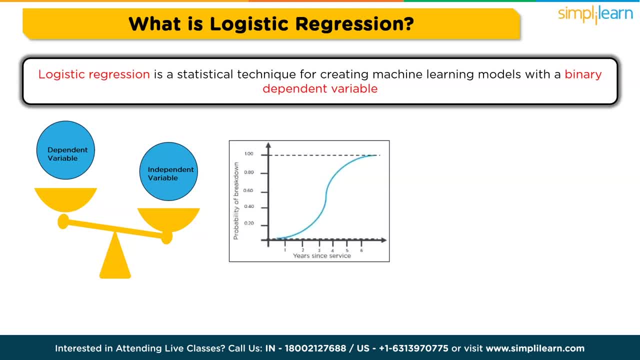 probability of a vacuole breaking down, depending on how many years it has been used since it was serviced last. So here is how you can interpret the result from the graph to decide whether the vacuole will break down or not. So, moving forward, let's see advantages of logistic regression algorithm. 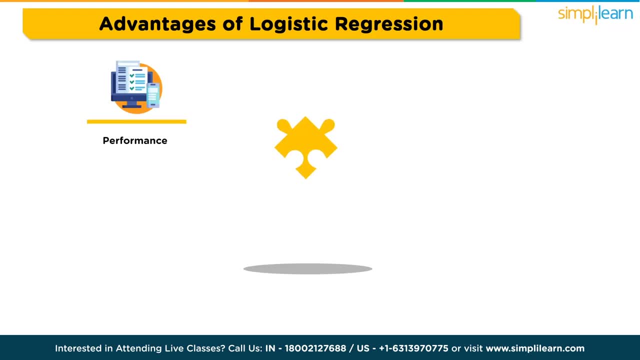 The first one is logistic regression performs better when the data is linearly separable. The second one is it does not require too many computational resources, as it's highly interpretable. The third one is there is no problem scaling in the input features. It does not require tuning. 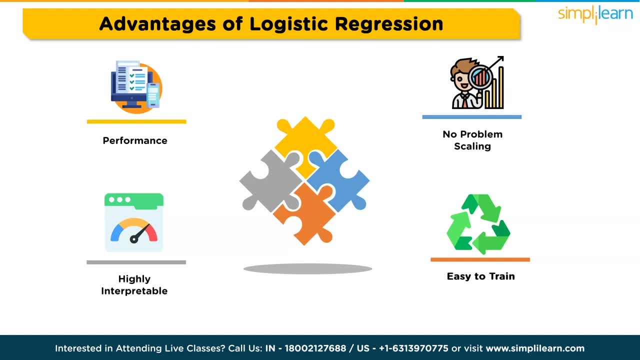 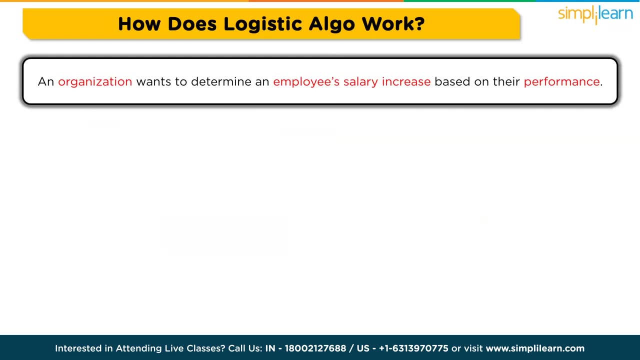 The fourth one is it is easy to implement and train a model using logistic regression. Now, moving forward, let's see how does a logistic regression algorithm works? Let's take an example. an organization wants to determine an employer salary increase based on their performance. For this purpose, a logistic regression algorithm will help them decide. 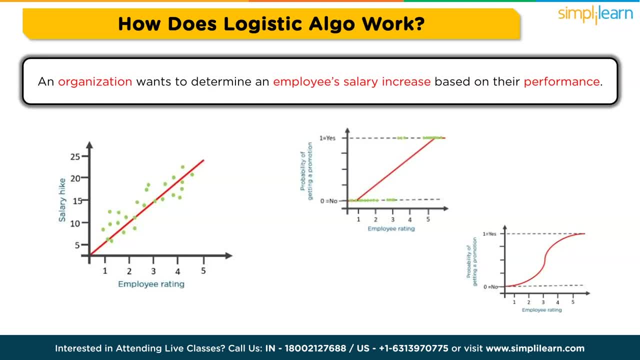 plotting a regression line by considering the employee performance as the independent variable and the salary increase as the dependent variable will make their task easier. So now, what if the organization wants to know whether an employee would get a promotion based or not? So the linear graph won't be suitable in this case as such, as we clip at the line at zero. 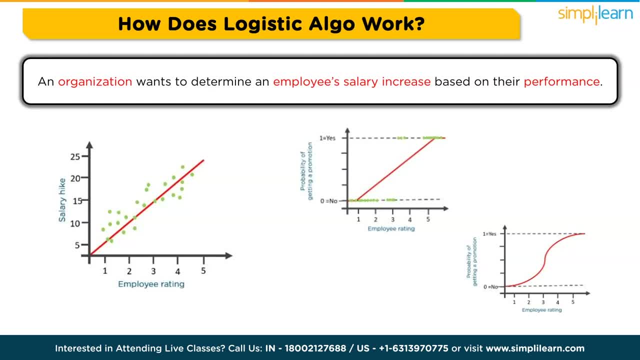 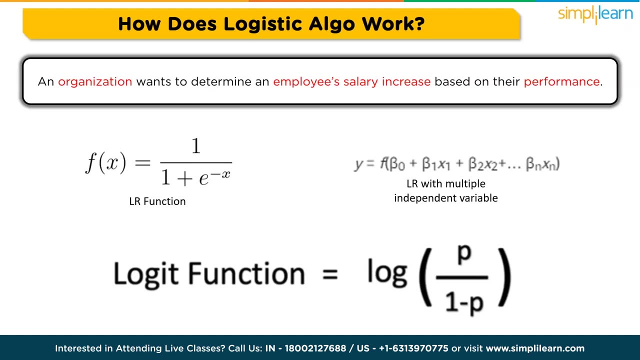 and one and convert it into a sigmoid curve s curve. So based on threshold values, the organization can decide whether an employee will get an salary increase or not. So there are some mathematical functions which can help you on finding logistic regression analysis. So these are some mathematical functions you can use in logistic regression analysis. 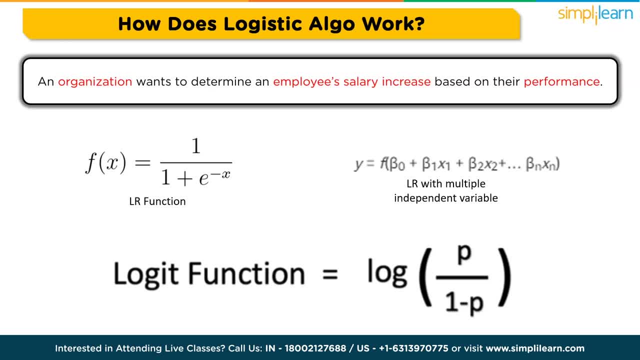 So LR function. Logistic regression is a statistical model that uses a logistic function or logit function In mathematics as the equation between x and y. so the logit function maps y as a sigmoid function. Logistic regression with multiple independent variable, In many cases multiple. 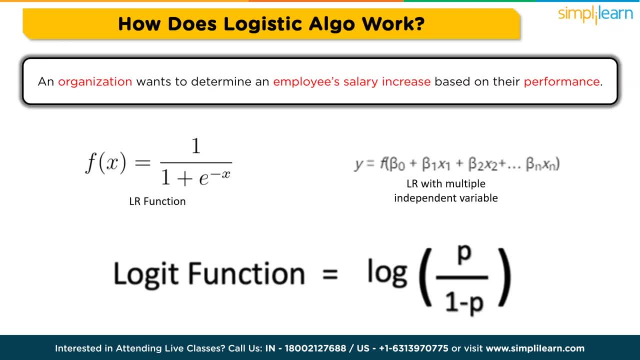 explanatory variables affect the value of the dependent variable Model. such input data set logistic regression formulas assume a linear relationship between different independent variables. So you can modify the sigmoid function and compute the final output. And the last one is the logit function. The logit function, you can also say the log odds, The logit. 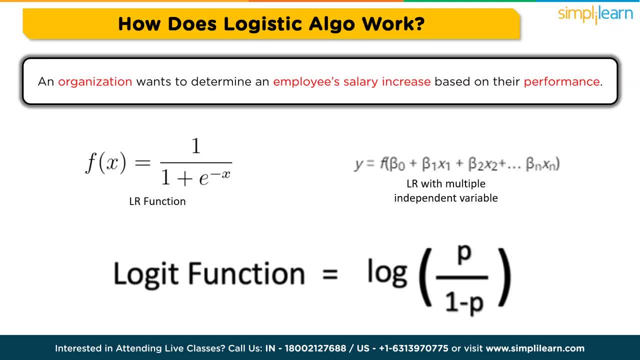 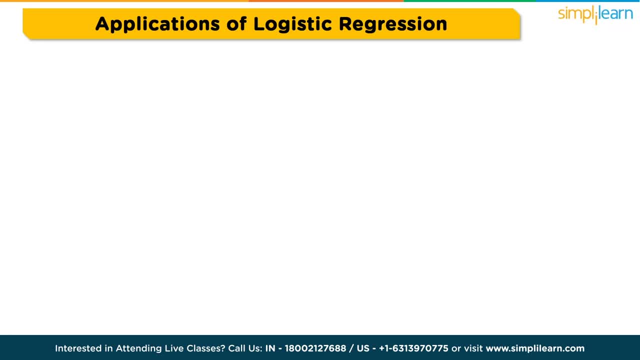 model can also determine the ratio of success to failure, or log odds. So, moving forward, let's see some application of logistic regression. The first one is banking. Using the logistic regression algorithms, banks can predict whether a customer would default on loans or not. The second one is to predict the weather condition or a certain place: Sunny, windy, rainy. 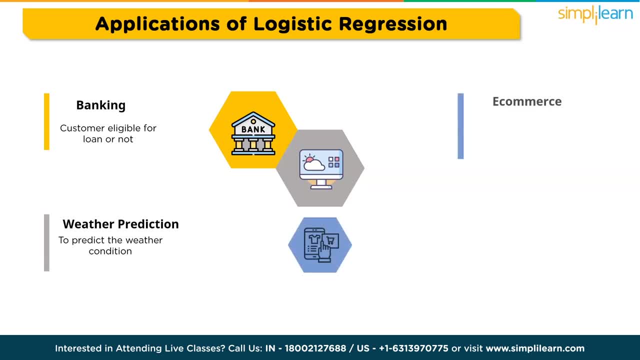 or humid you can predict from logistic regression. The third one is e-commerce. E-commerce companies can identify buyers if they are likely to purchase a certain product. The fourth one is: companies can predict whether they will gain or lose money in the next quarter, year or month based on their current. 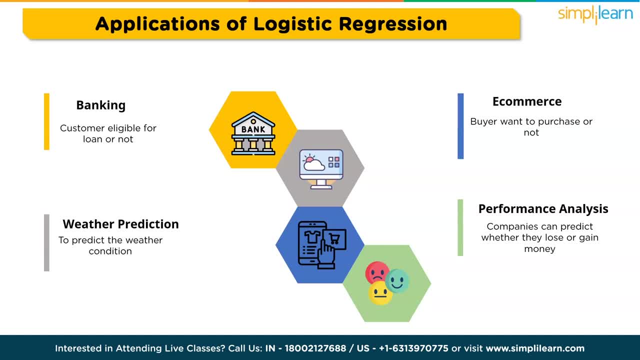 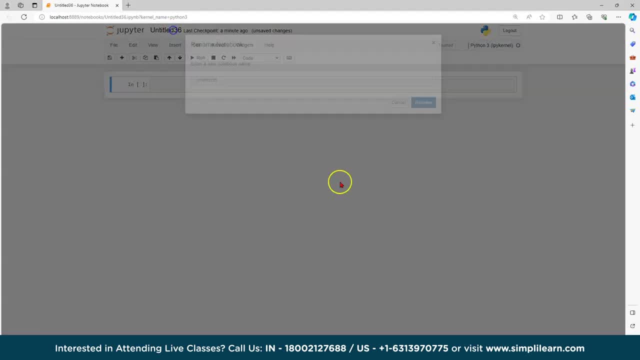 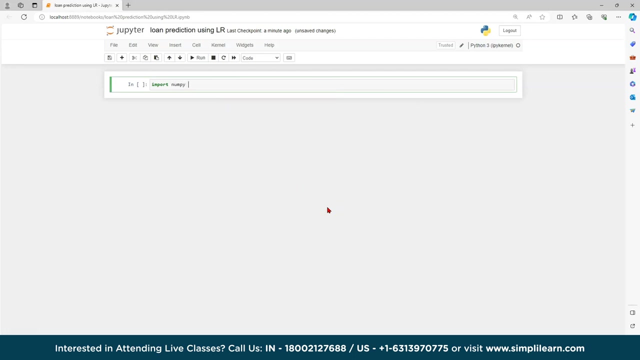 income. So now, moving forward, let's jump into our Jupyter notebook to implement logistic regression demo. So now, here we will do loan prediction using logistic regression. So first I will change the name: loan prediction using logistic regression, right. So we will import some major libraries like numpy: import numpy as np and import. 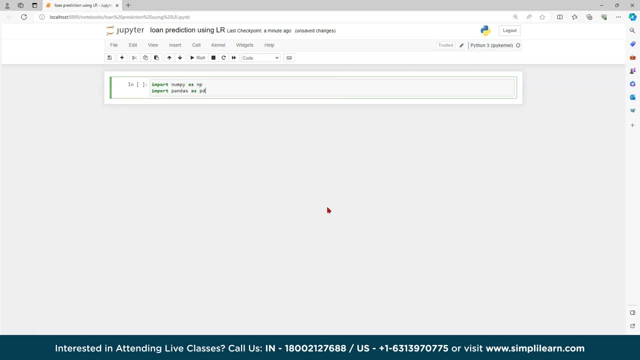 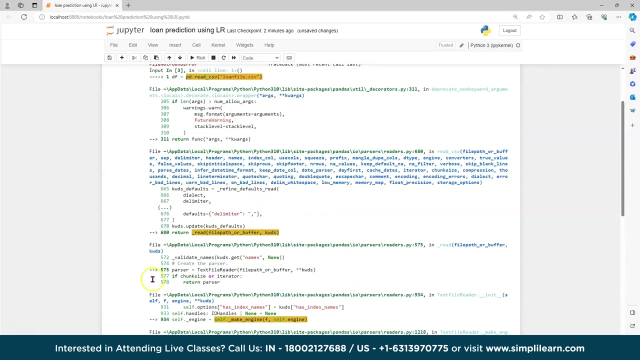 pandas as pd, then import matplotlib dot. pysplot as plt, then we will import seaborn as sns. So moving forward, we will import one data set, ed dot. read underscore: CLомуn CSV. okay, spelling mistake okay. okay, let me check the file name first. so a file. 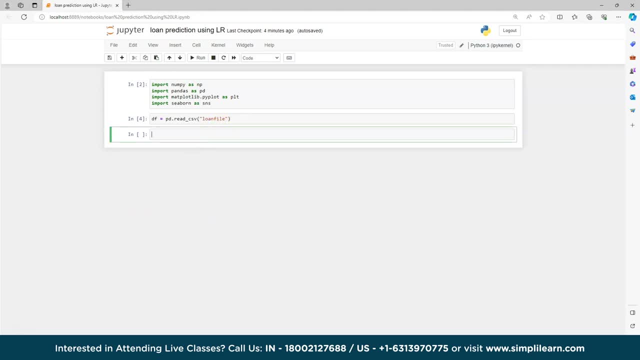 name is loan file, so moving forward we will lose some function. let's check. so this is our data side. so in this there are like multiple columns: name, loan ID, gender, marry dependents, education. this is then. let's check the info of the data set. we have taught info. 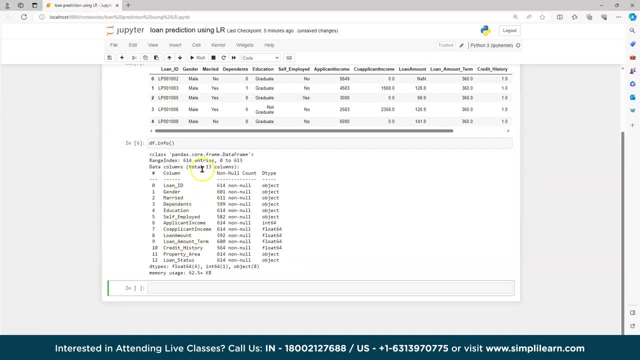 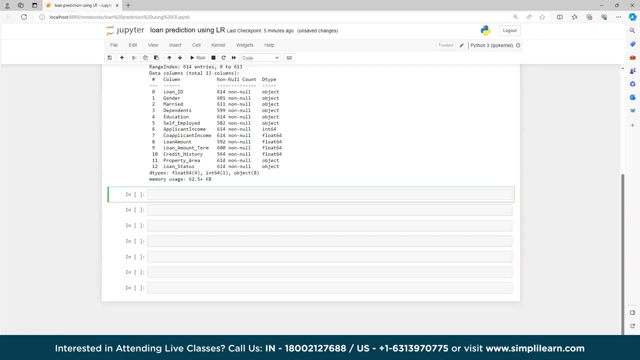 so, as you can see, so we have 13 columns, right, total 13 columns, and the column type is this: object, object, float and object. okay, the memory usage and all. once again, let's check how many rows you have: dog shape. so, as you can see, we have. 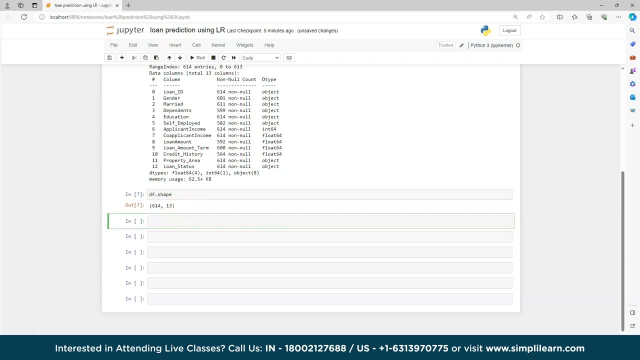 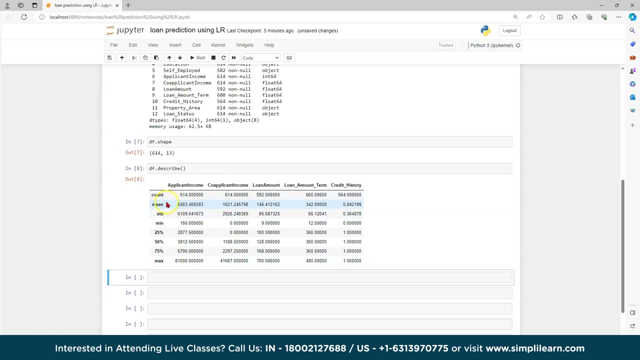 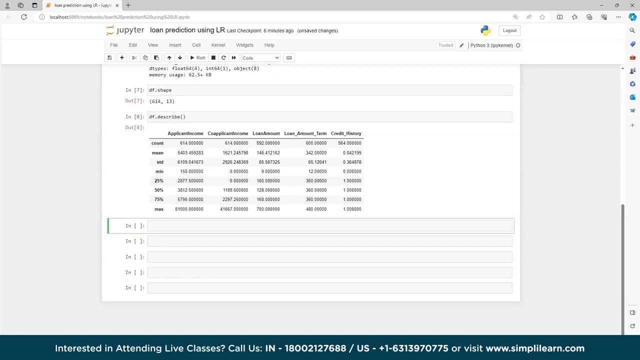 614 rows and 13 columns present in our data set. okay, we'll check. describe as well. yes, so this is the count of the particular column: the mean, then the standard deviation: minimum: that 25 percent of particular column. okay, the maximum value: the 75 percent of the particular column value. okay, let's check. 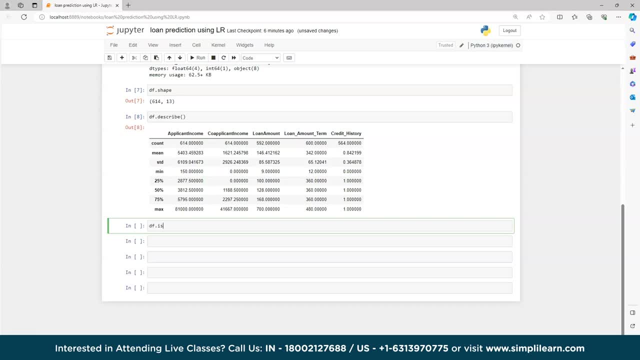 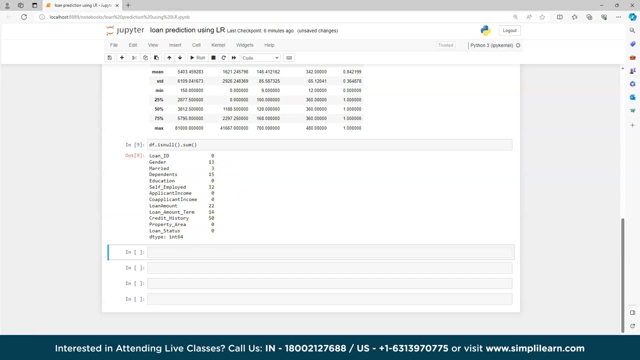 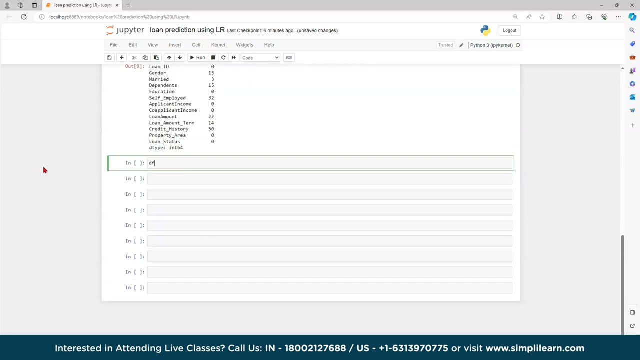 how many null values are there? so for that, right this now, because first we have to sort what data set for the better predictions. so loan id don't have any null value. gender: have married: okay, right. so now let's do some data cleaning here. for data cleaning, we'll write df. loan amount equals to df. 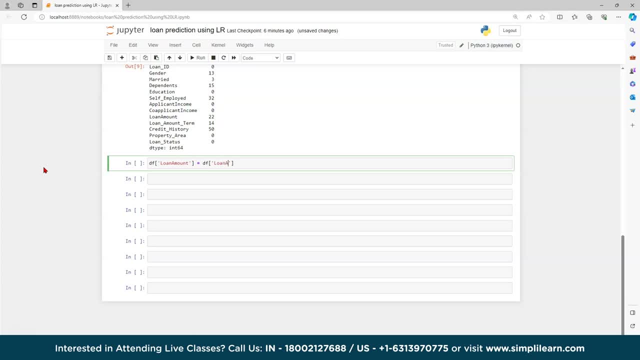 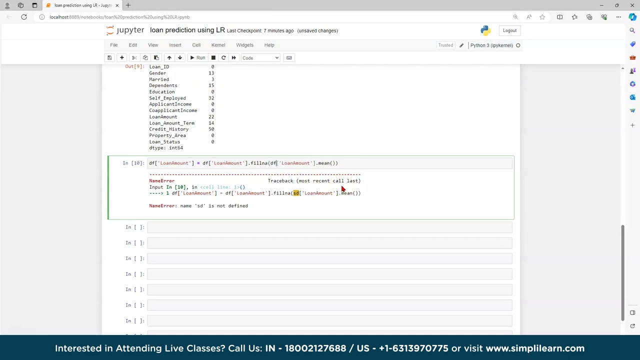 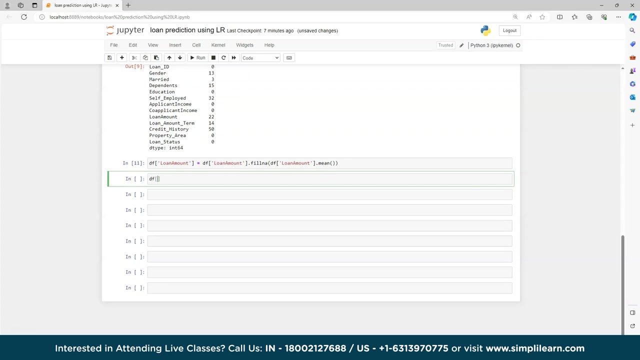 df loan amount. dot fill na okay, df loan amount. dot mean: okay, df, right. so for credit history we'll check df, then get it straight. so i'm filling the particular cells with the median or mean values, okay, then df credit history: again straight: dot median, right. so now again let's check this nine dot sum. 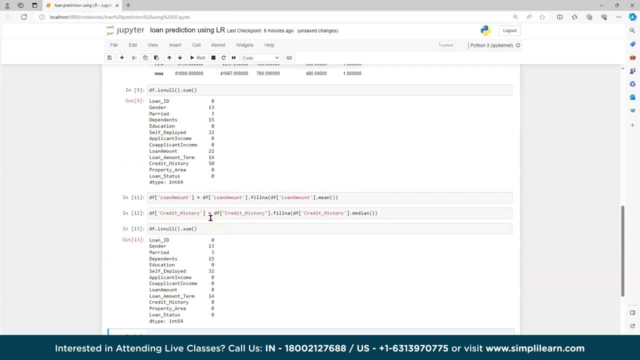 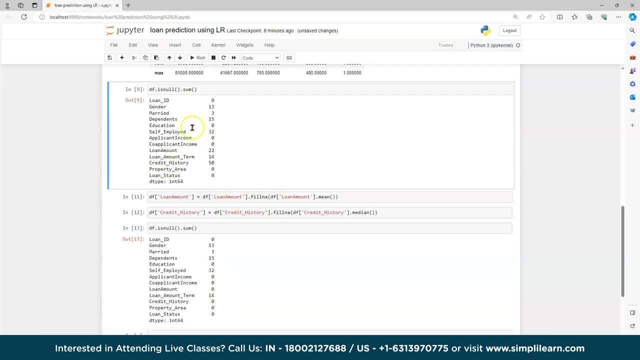 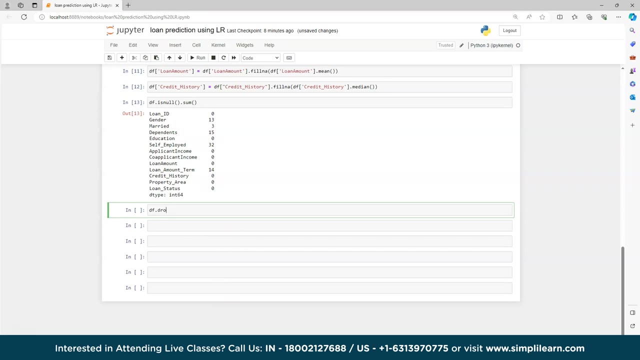 okay, fine, cardistry, now zero. as you can see here, you can see the carrier history is 50, 15 l values are there? now zero. and one more loan amount: okay, 22, now loan amount is zero. so df dot drop n place equals to true. and now df dot shape. 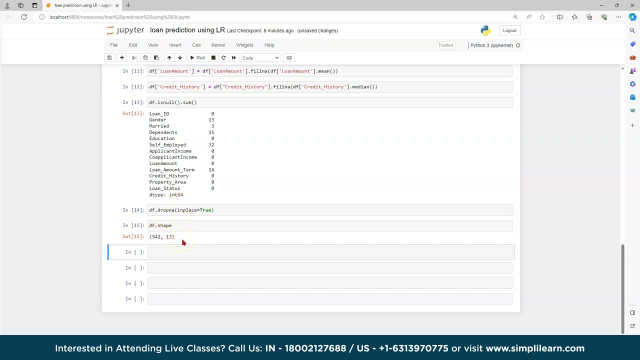 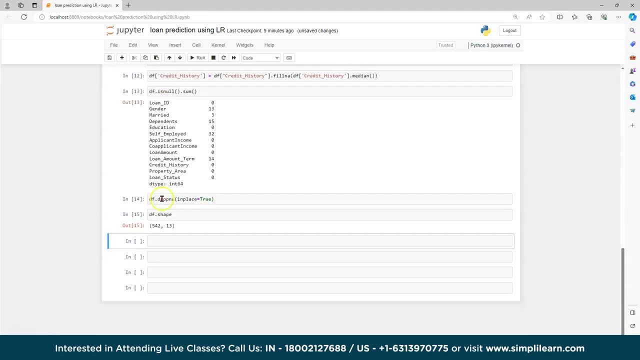 so now, as you can see, we have dropped the all the uh, you null values rows. as you can see, the 542 here before it was 640, right. so now let's moving forward. we will do some eda, okay, some data representation. so here what we will do: we will plot some graphs, right, so i will write a plt dot. 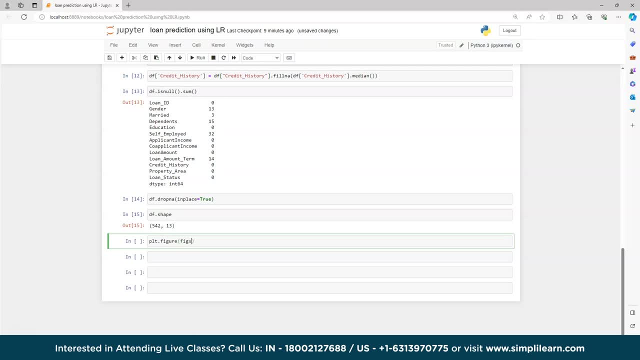 figure. then figure size equals to 100 comma 50, then sns dot set font scale equals to 5 plt dot subplot 331. sns dot count plot, then df. where i need gender, then hue will be df, then loan status df. right, so i will do the same for the married and the education, then the self-employed. 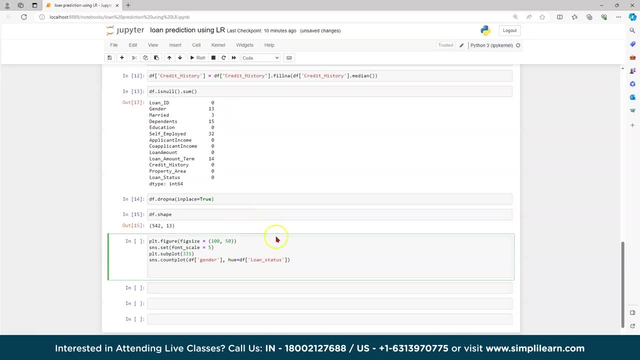 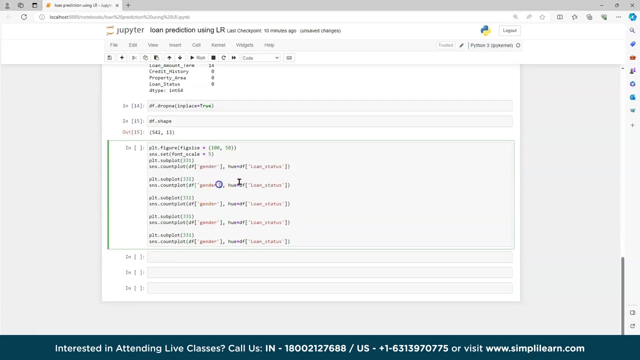 then the property area. right, so i can copy this and paste it here. right, one more i need. okay, then i will change the name. but i need married who is 32, d33 for education, 364 Phone, 34, 4 uploaded. but I will do one more thing. 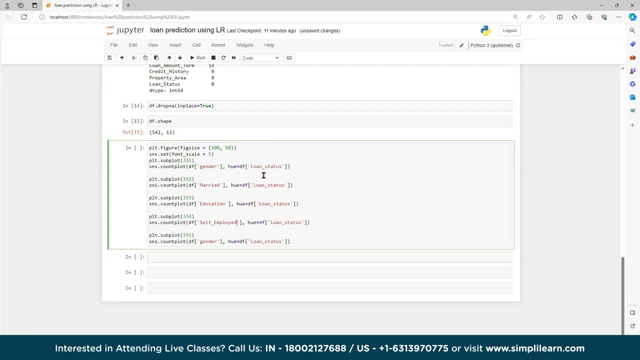 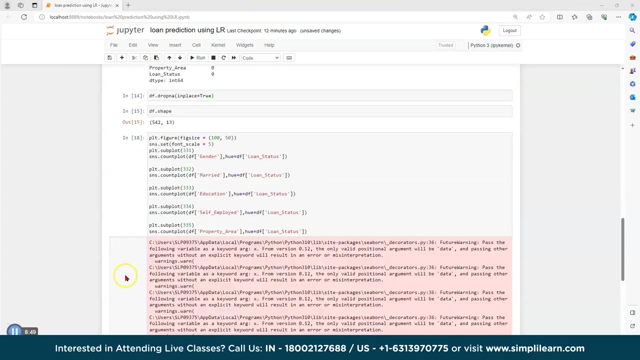 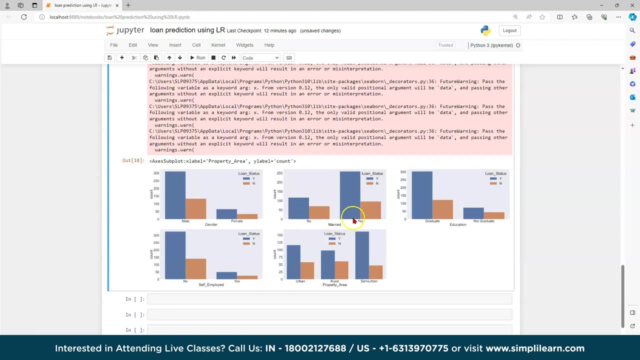 Which is They? I think some of them. they may answer this question today. one more question: go ahead and type information in there. go ahead and do it right. okay, let's run it, it's loading. so now, as you can see, these are some bar graph like: how many married are their loan status yes or no? the blue one is: 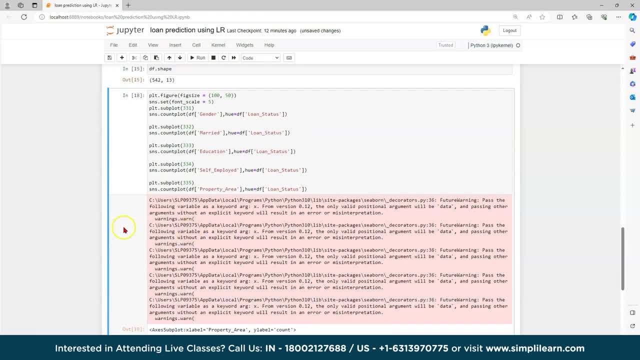 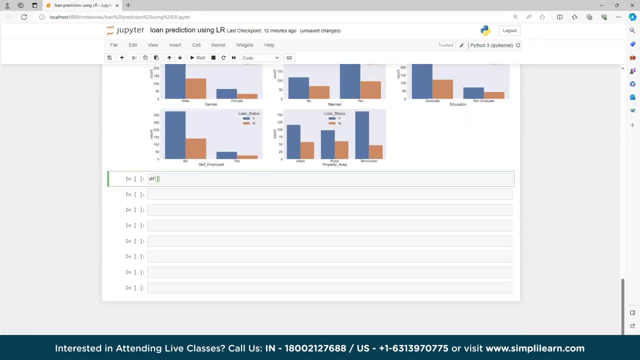 yes, okay for the education, for the self-employed. so these are some warnings. you can ignore them right? so moving forward, we will check some loan status, so I will write here: I want only loans status. dot replace y to 1 and n to 0. okay, so later it will be good to check comma 1 in place goes to true. same for. 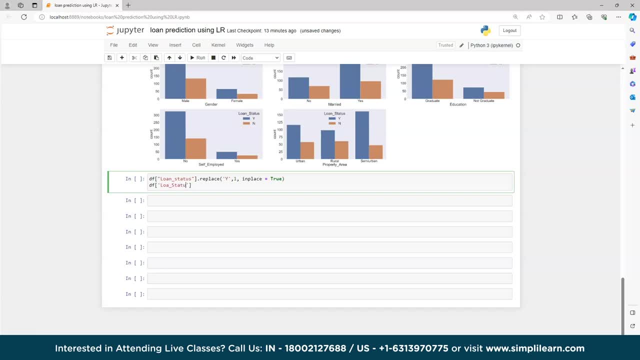 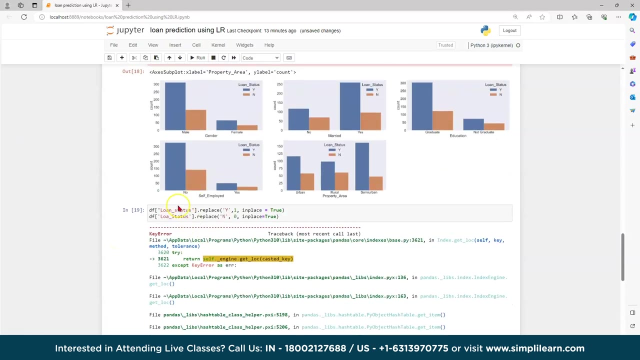 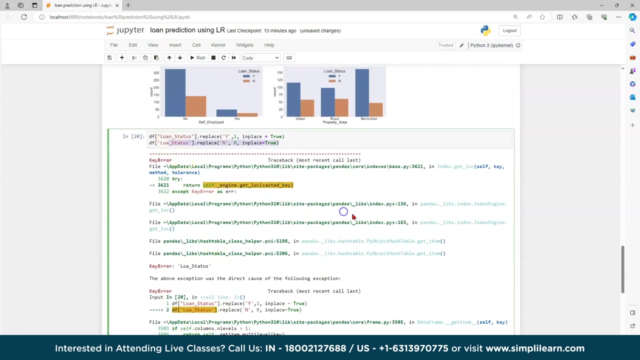 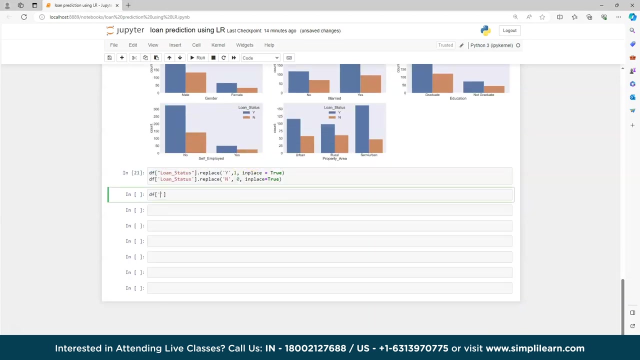 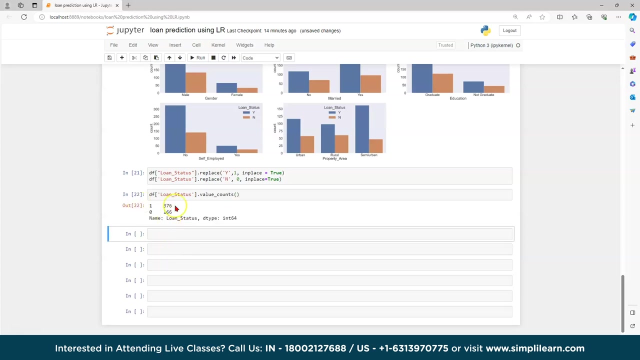 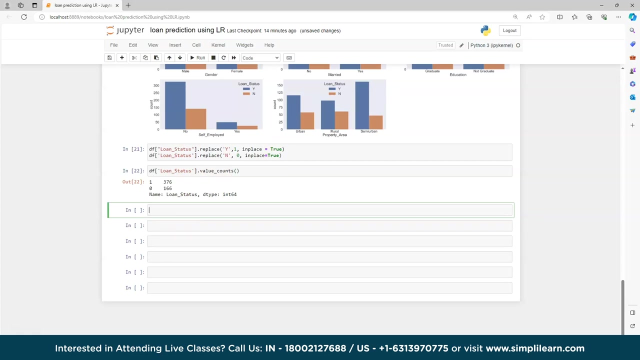 no status dot. replace n comma 0 comma n place goes to true. okay, loan status s is capital here. okay, it is nothing, just a typo mistake. okay, so here I will write df, status value, count value. okay, so yes, r376 and no R166. right, so we'll. 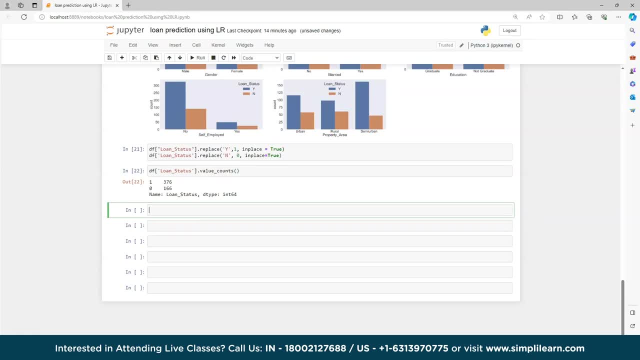 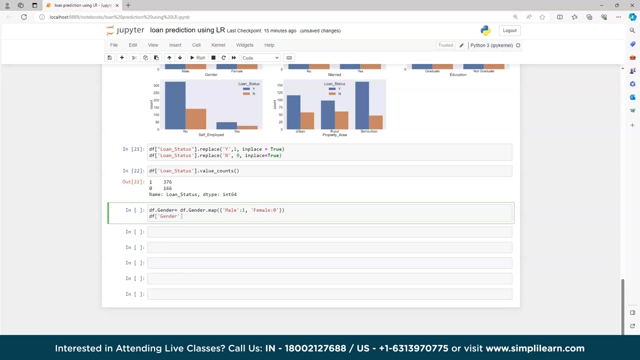 check with the gender, married and dependence. okay, so for that I will ignore df dot gender equal to df dot. male. Request to df dot gender. G is capital here dot map. then male is 1, female is 0,. right, Then I will write df gender dot value counts okay. 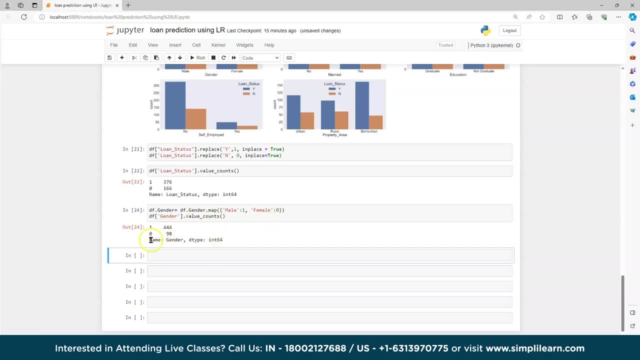 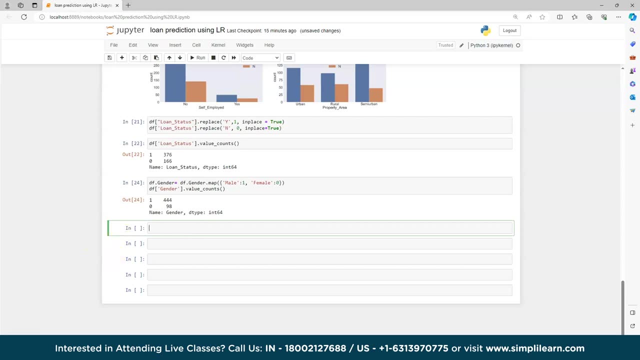 So now I gave male to 1 and female to 0,. okay, So this is the gender count, right? So I will do this for Mary, Mary, as well as the dependents. okay, For all the education. self-employed property area: okay. 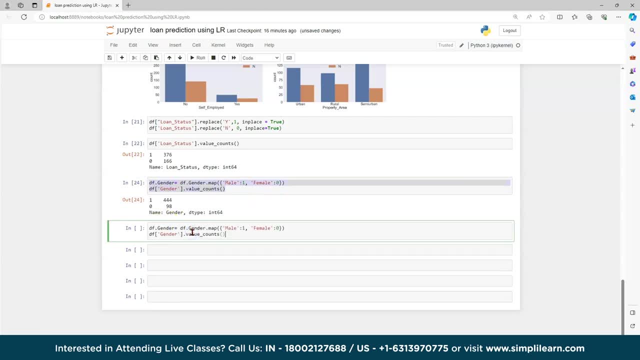 So what we can do, we can just copy it, paste it here and we can change right. For the Mary married for yes to 1.. So let me do it fast for you and then I will get back to you. 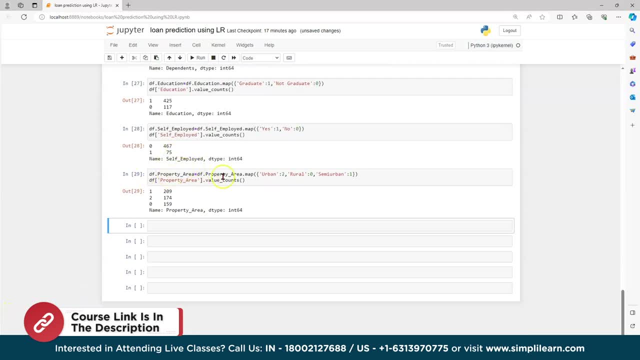 So, as you can see, we have done with the. all the value counts here, like property area, self-employed, education, dependents, married. okay, We have all the counts. So now let's see the loan amount value count. loan amount- dot value counts. 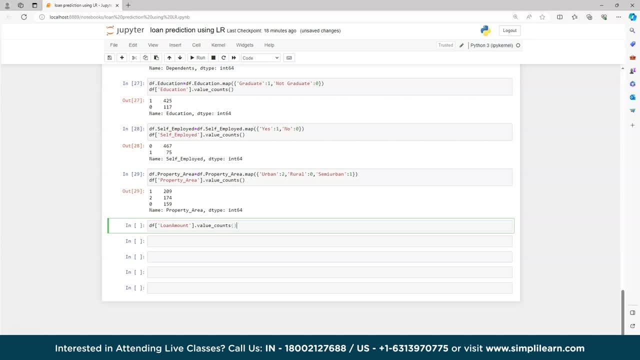 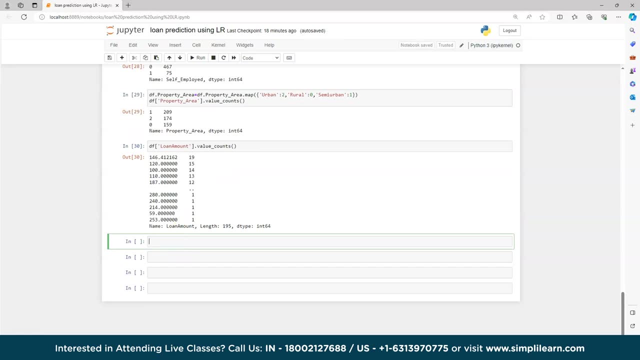 Okay, Okay, Okay, Okay, Okay, Okay. So this is the loan amount value count. then we will check the loan amount value term. For that I will write loan amount term, dot value counts. right, Then let's check the credit registry, which is very important factor for the loan. 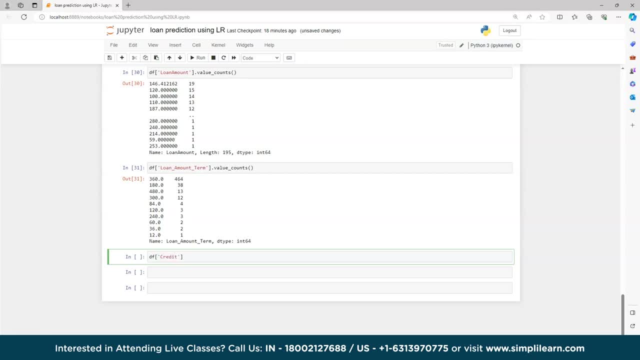 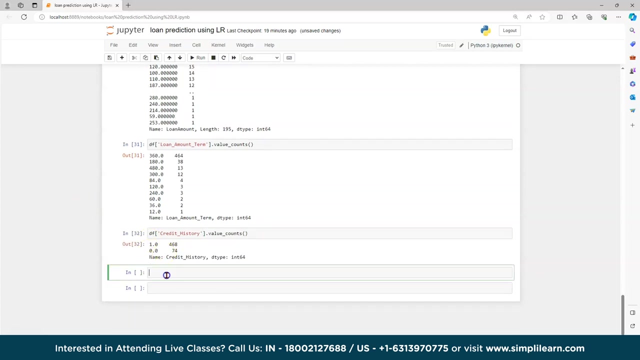 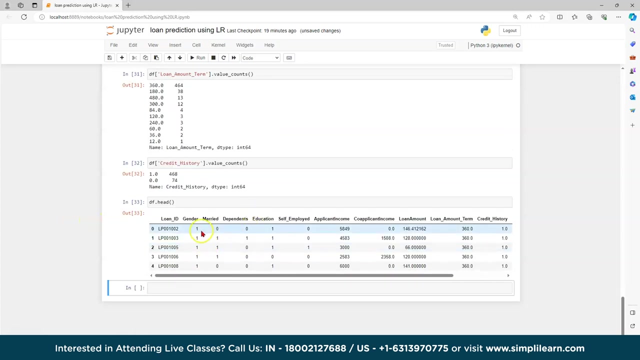 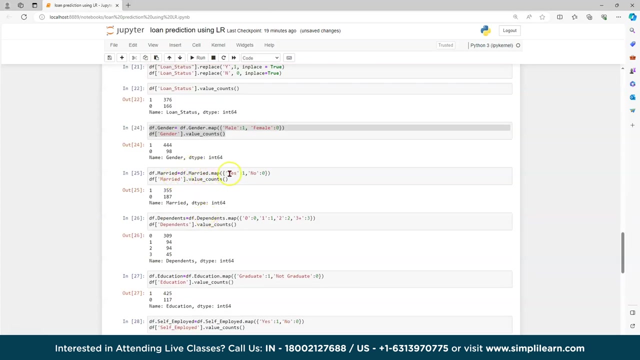 Okay, Okay, Okay, Credit history dot value counts, okay, Right, So now let's check df dot head. Okay, Okay, as you can see, we have this. see, one means male. here you can see we gave married the gender male. 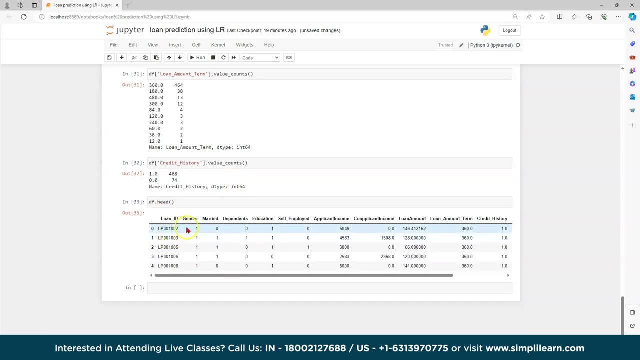 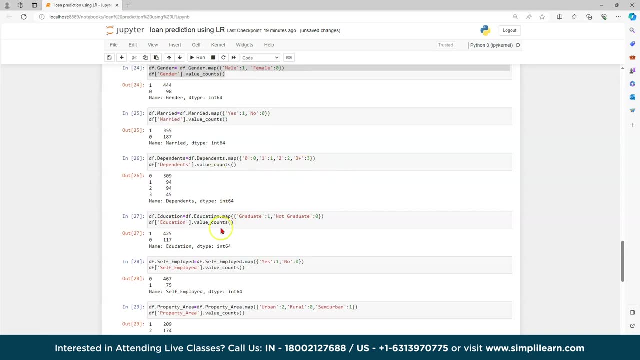 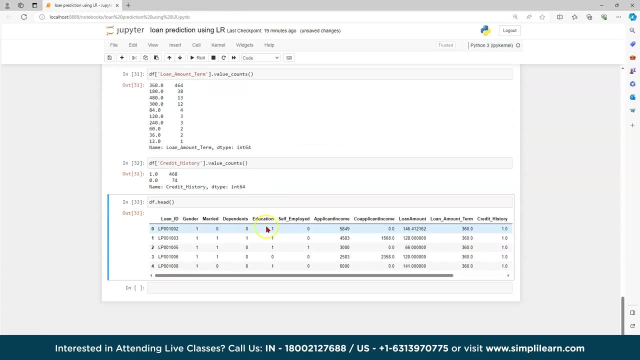 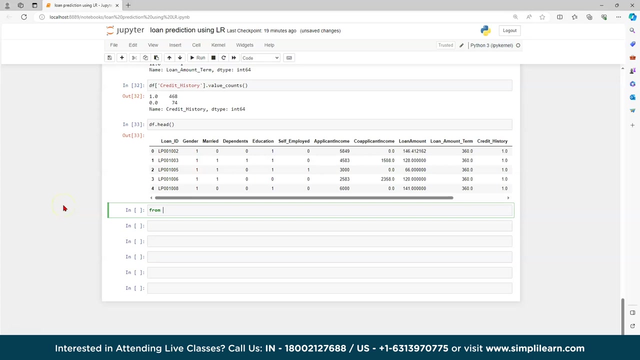 equals to one, then female is zero. so this is this id. is male id, right, then zero one. we have all gave here like zero one, zero one, right. if the guys graduate, so one, not graduate, so zero. sam employed is yes or no, like that, right. so now we'll do the train test split, okay, for that i will write from: 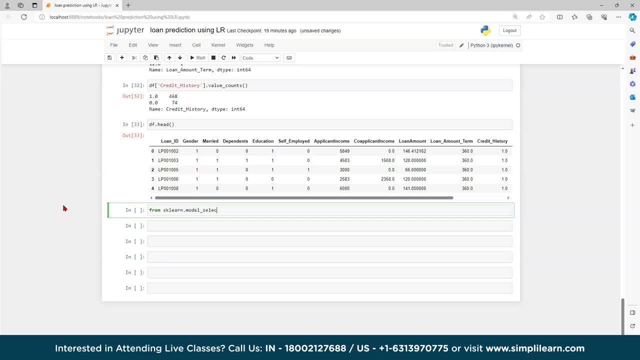 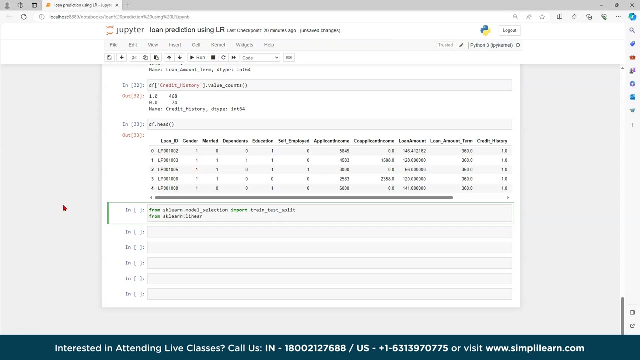 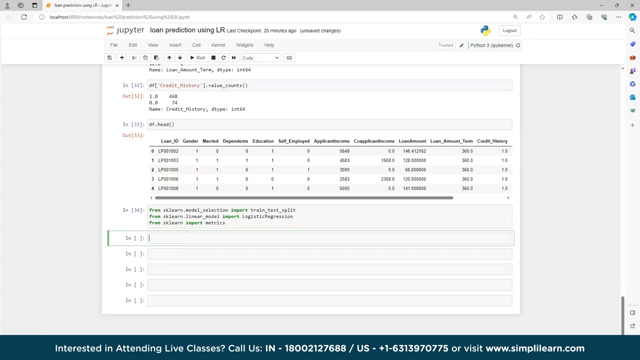 sk learn dot model selection: import train test. split then from escalon dot linear model logistic regression. okay, then i will write from skill learn import matrix. okay, let me run it. so here i will assign x equals to df dot. i log then one ratio: 542 rows, then from one. 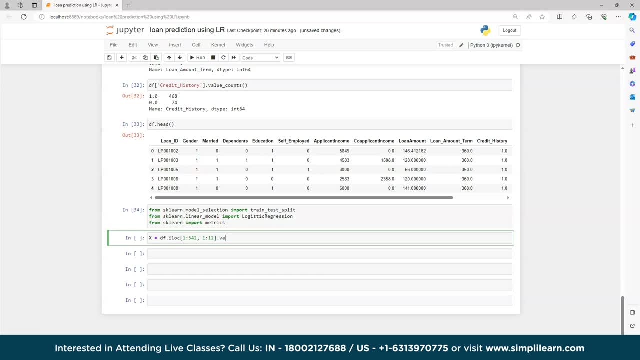 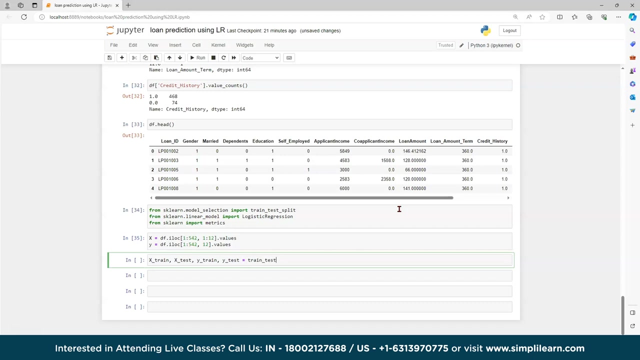 to twelve columns dot values. then y equals to df dot. i log the same, okay, one, two, five, forty two rows, then called dot values. okay. so here i will do x train comma, x test train comma, y test equals to train test split. then x comma, y comma test size equals to 0.3. 0.3 means seventy percent will be the training data. 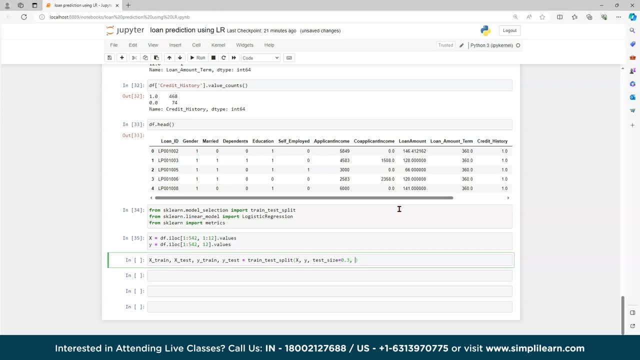 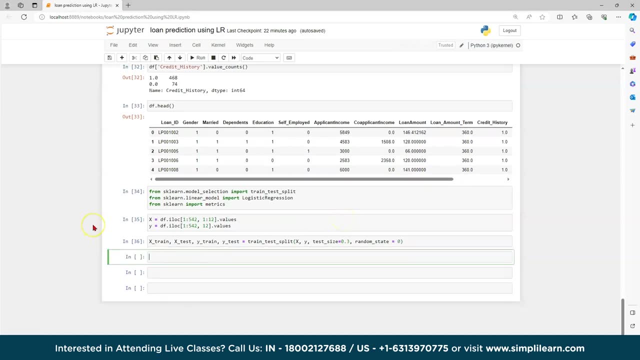 and the thirty percent will be the testing data. right, random state got it. so now let's do the logistic regression. let's apply model goes to logistic decoration, then model dot fit X train, Y train, then LR. let's go prediction, because model don't predict the next test. right, then print logistic. 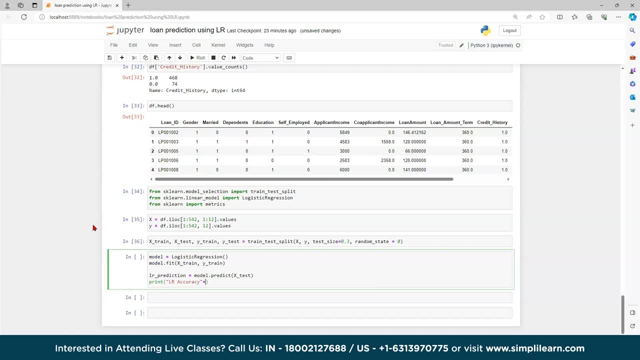 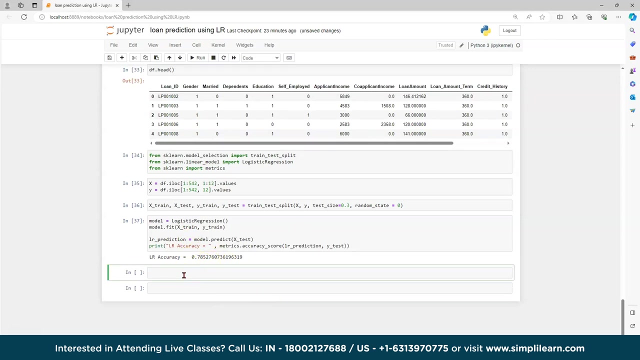 regression accuracy goes to comma matrix dot accuracy underscore score. then I will write LR predictions, comma Y test, right. so as you can see, we have the accuracy of almost 79%, or you can say 78%, right. so now let's see the predicted values. so for that print Y prediction, predicted value. 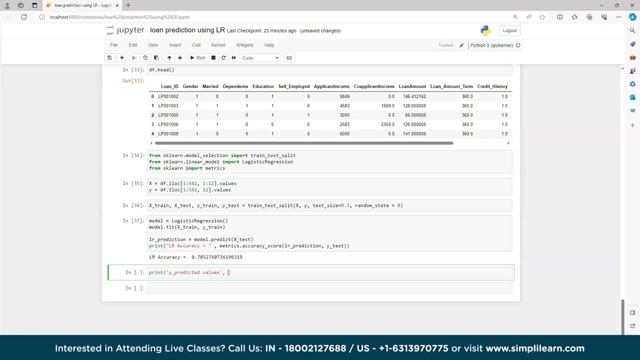 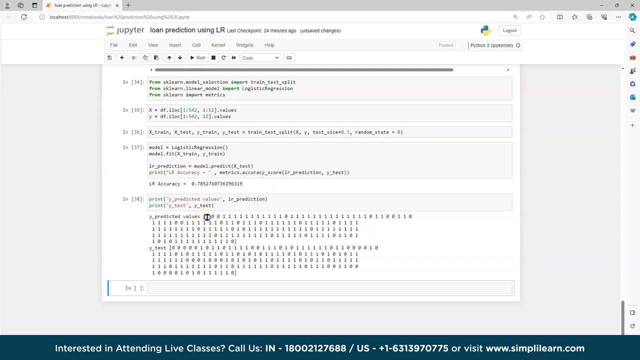 values: comma: LR prediction: okay, used in our model test. LR condition: okay, then print Y test: um. why less test? so, as you can see. so these are some predicting values like one means that guy or girl have the loan. okay, loaning status is yes. loan prediction status is: yes, then zero means no like and the testing we did, the hair: zero. okay, the pi valuable Ahab's researchcountry values one right. so these�� regimentation b4, 2018, 2020, 2020, 20th kind of ç be false funds in me. wasicestations, cx60, everybody in this training series. community 1240, 6可以丸視回에게. 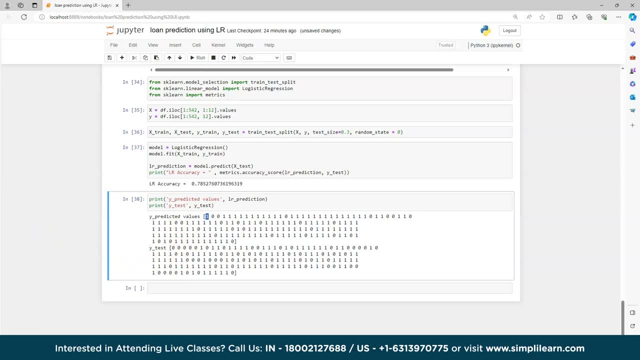 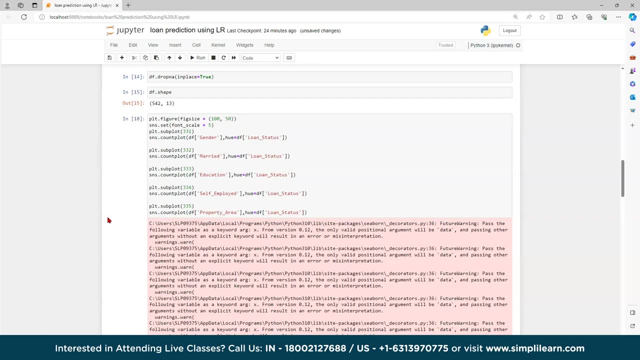 are some prediction values and the testing values. so this is how you can do loan prediction using logistic regression. okay, so we have come to end of this video. if you want this full code, you can comment down below and if you want this file- loan file- so you can check out from the description box below. 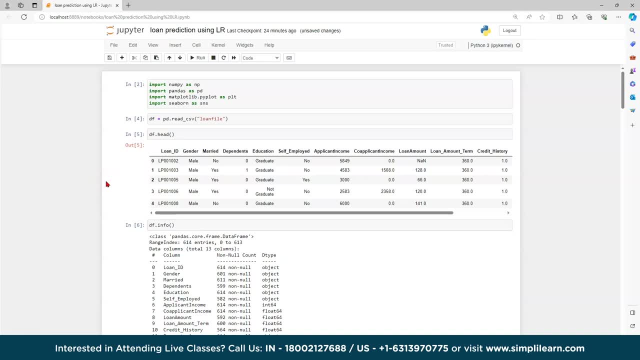 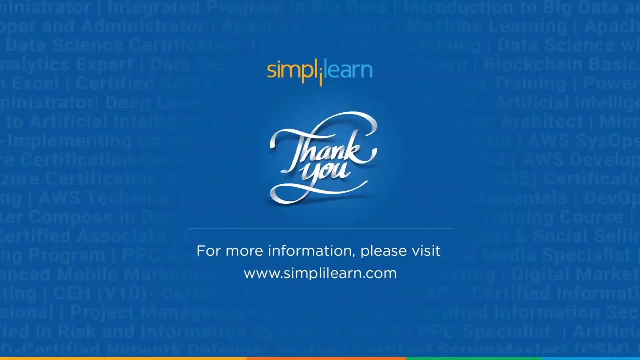 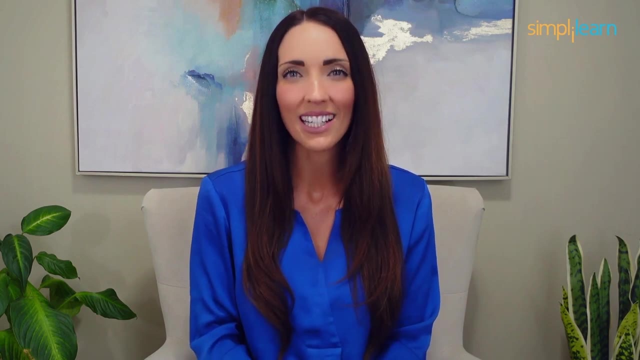 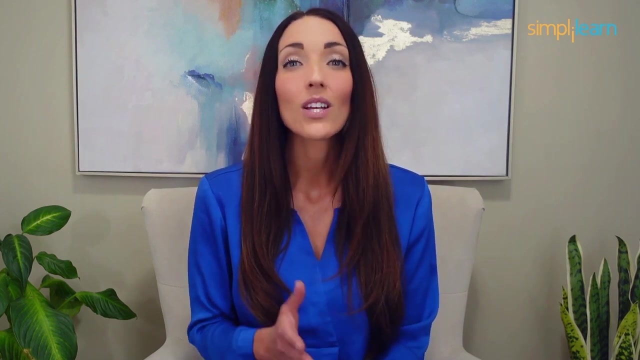 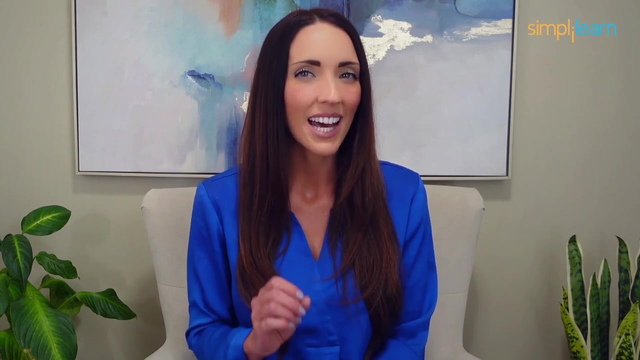 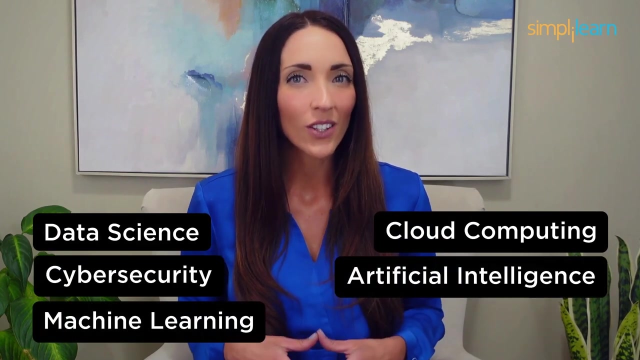 and if you have any queries, so please comment down in the box. we will reach out you as soon as possible. thank you for watching the video. please do like, share and subscribe. thank you and keep learning with SimpliLuv, or digital marketing Designed in collaboration with leading universities. 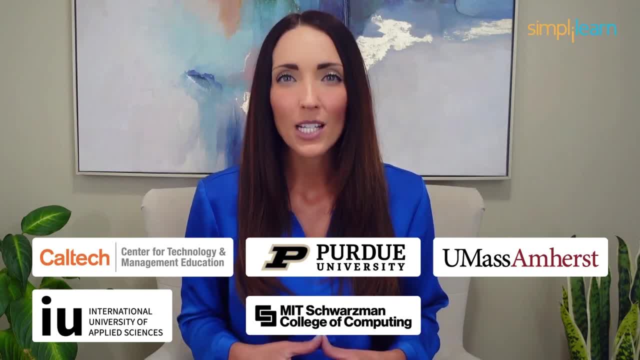 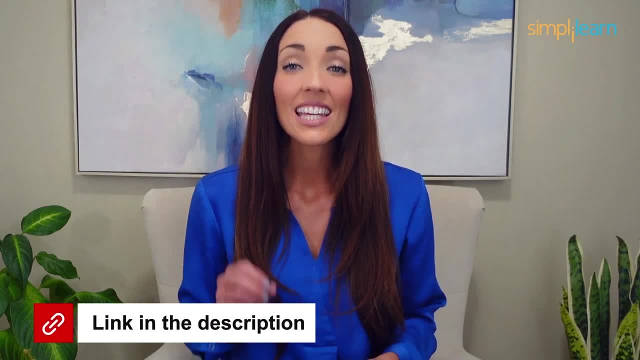 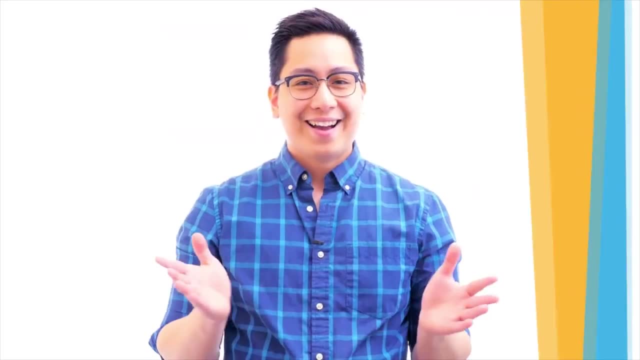 and top corporations, and delivered by industry experts. choose any of our programs and set yourself on the path to career success. Click the link in the description to know more. Hi there. if you like this video, subscribe to the Simply Learn YouTube channel and click here to watch similar videos. To nerd up and get certified: click here.